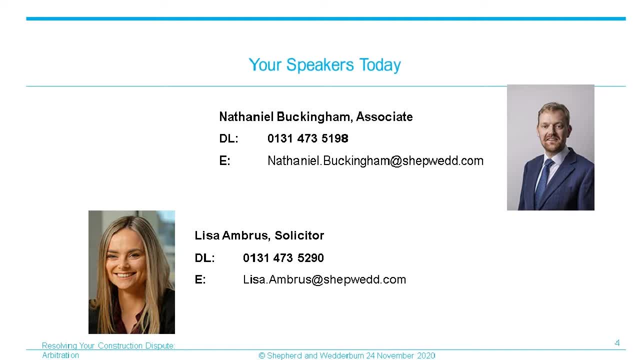 a solicitor in our team. Our team regularly advises on construction contract issues and disputes across a range of projects and clients. We therefore will be answering your questions at the end of the presentation. If you have any questions, please do so by using the ask a question tab. 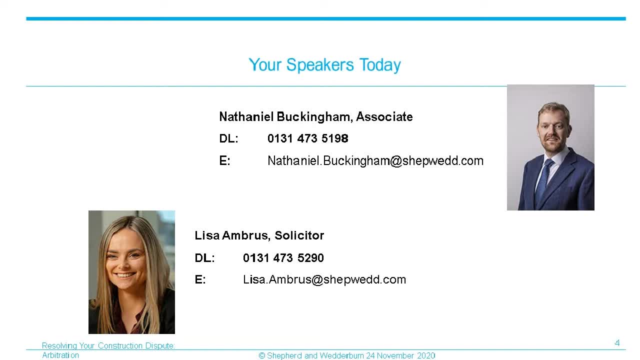 If you have any questions, please do so by using the ask a question tab. We therefore have a great deal of experience in litigation, arbitration, adjudication and mediation, where our arguments have to reflect ever evolving judicial approaches to construction law and contracts. So I will now pass you over to. 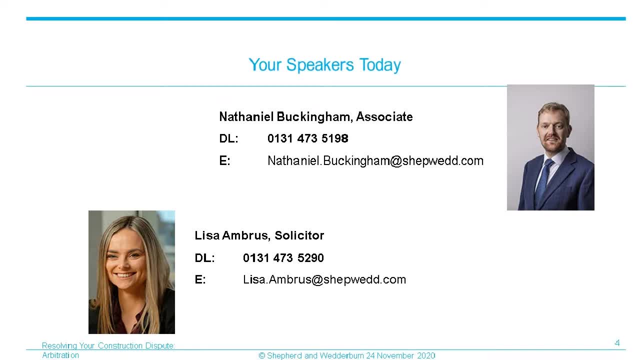 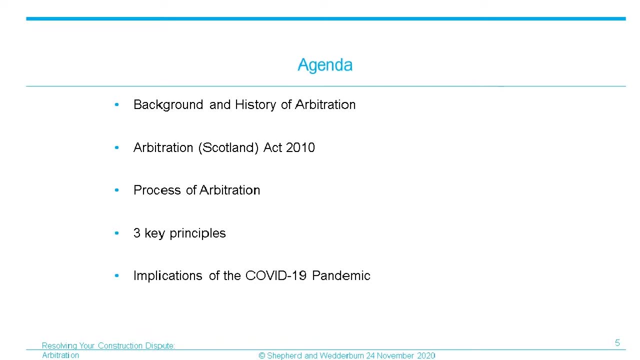 Lisa, who will run through the agenda for today's webinar. Thanks, Nathaniel. We will begin our presentation today with a brief overview of the history of arbitration, before moving on to discuss the introduction of the arbitration and how arbitration is practised under the auspices of the Act. We will highlight the three key. 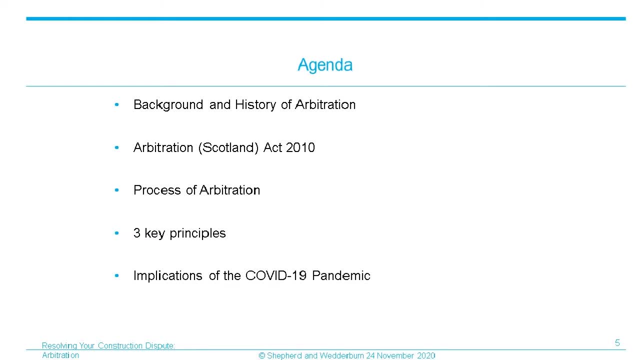 principles which guide arbitration and explain how they are reflected in the current governance structure. We will then discuss how arbitration has responded to the current remote working environment. As with many of our other webinars, we primarily deal with Scots law, and more specifically the Scottish Arbitration Act in this session. 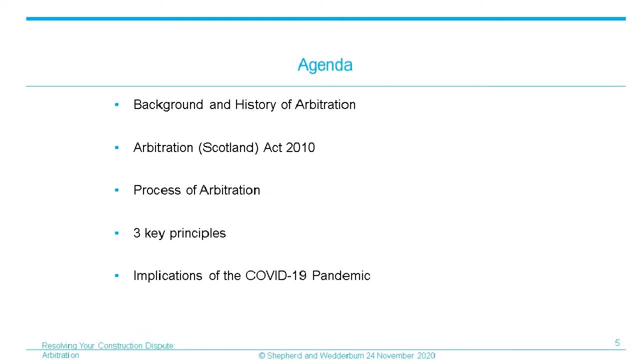 We will also discuss the position of the Scottish Arbitration Act. in England Much of Scots and English contract law and many of the standard form contracts used for construction projects are common both sides of the border. We advise on both Scottish and English disputes regularly. But before all of that, the first thing we should cover is what arbitration actually is. 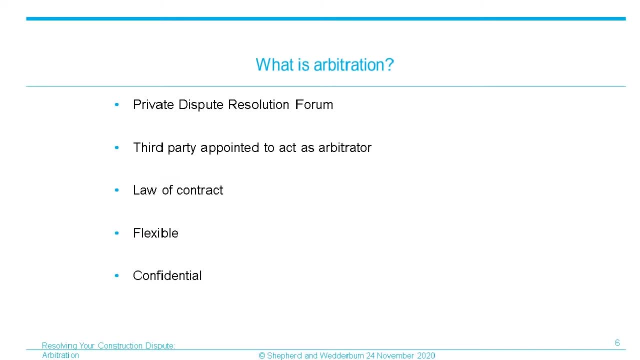 So arbitration is a private dispute resolution forum which is often employed as an alternative to court vieced over by court Pr Vanessa ss the dispute court. The parties to the dispute appoint an arbitrator to act as a judge who reaches a decision that is binding on the parties. Alternatively, the parties can also appoint a panel of arbitrators, known collectively as the Tribunal. The terms are used interchangeably. Arbitration is based on the law of contract. The Arbitration agreement is what gives the arbitrator jurisdiction to decide on the dispute. It is by this Arbitration agreement that 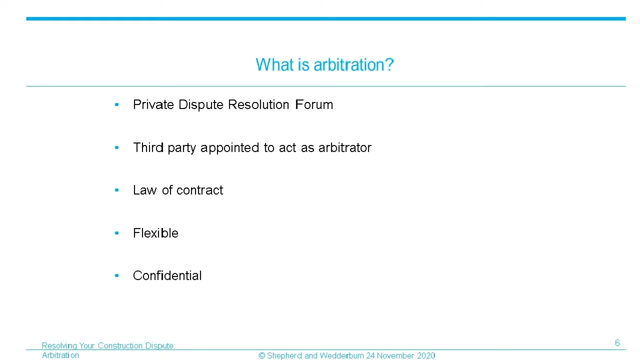 there is essentiallyЕН accordance that the parties are bound to follow that decision. This is a distinguishing feature of arbitration, which can be seen when we compare it to other forms of dispute resolution, For example mediation, in which the third party is there to assist the parties in coming to their own decision. 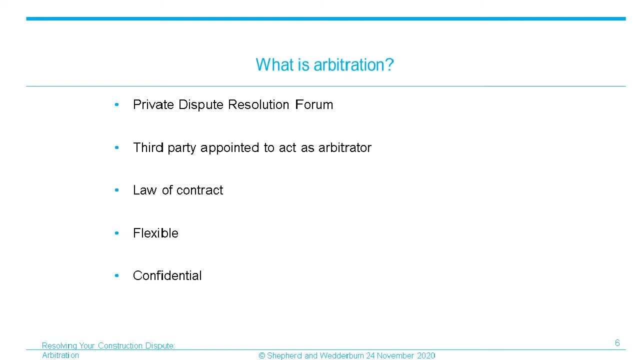 Arbitration is an attractive option due to its flexibility. The procedure can be adapted to suit the parties and their dispute Parties also favour arbitration as it is confidential, which can be beneficial where the dispute is commercially sensitive. An arbitration award is final and binding on the parties. 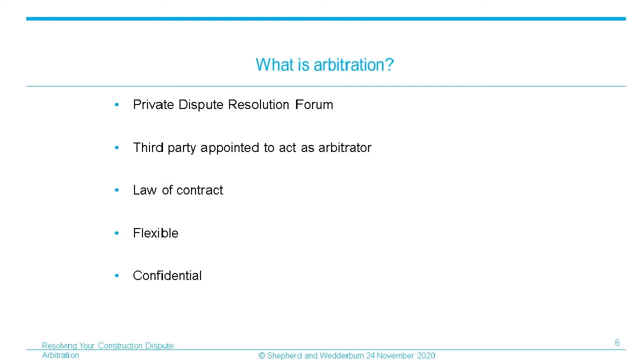 and cannot be challenged except on very limited bases. These are a lack of jurisdiction, a breach of natural justice on the part of the tribunal, or appeals on errors of law if the default rules are applied, which we will discuss later in this webinar. So historically, arbitration in some form was practised in Scotland. 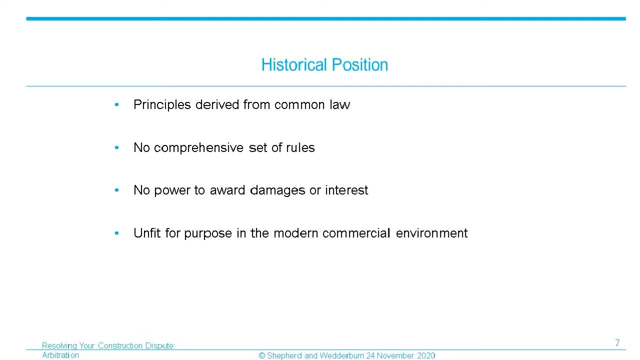 before the public courts were established and has since continued as an alternative to litigation. Until relatively recently, arbitration was conducted under judicial principles derived from cases in the 19th century, which were occasionally supplemented by legislation on specific aspects of procedure. The law was patchwork and difficult to understand. 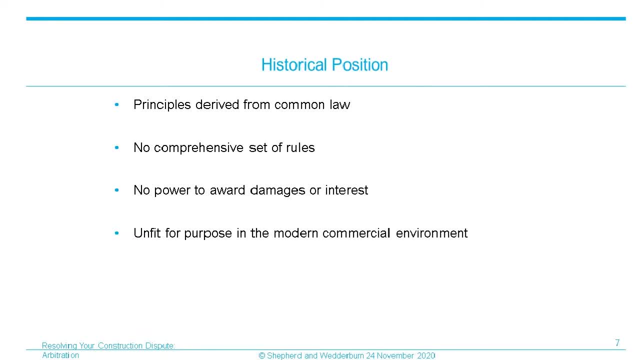 and in the absence of a comprehensive set of rules, too much was left in the hands of the individual parties to the dispute, and this often prevented arbitration from being an effective way of settling any dispute. The arbiter, as they used to be called, also lacked many of the powers which they are now granted, For example, an arbiter. 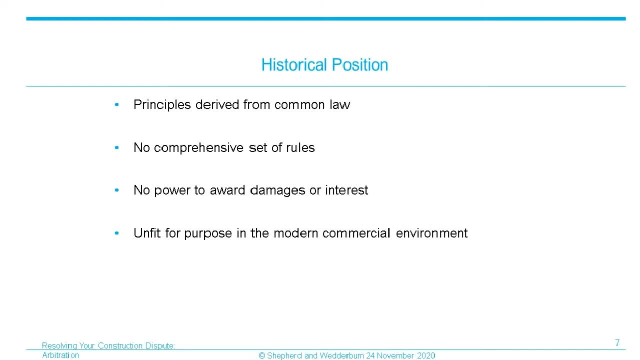 had no power to award damages or to order payment of interest on any award. This latter deficiency was especially problematic as arbitrations could last much longer than they do now, up to eight or ten years in some instances. It is clear to see that this framework was considered unfit for the 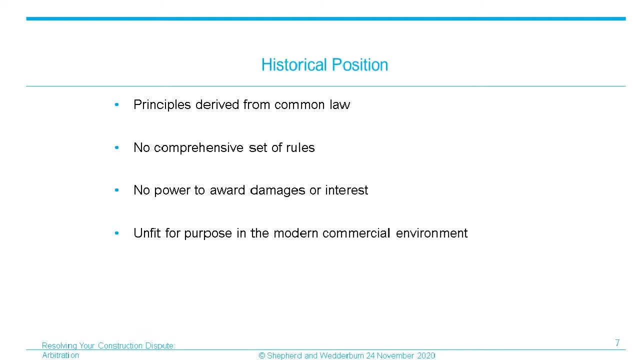 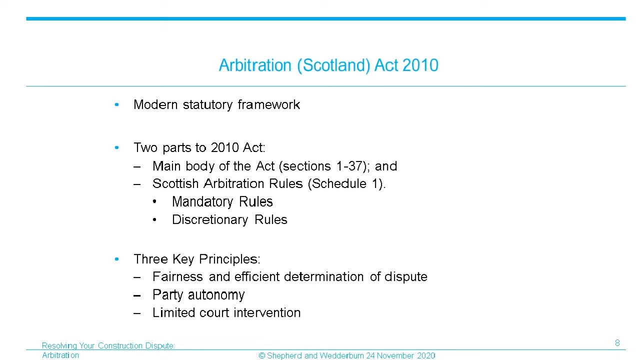 modern commercial environment. Arbitration became so unpopular that in 2005, the Scottish Building Contract Committee removed arbitration as the default method of dispute resolution from its standard form: construction contracts. These days, arbitration is governed by the Arbitration Act 2010.. This provides a modern statutory 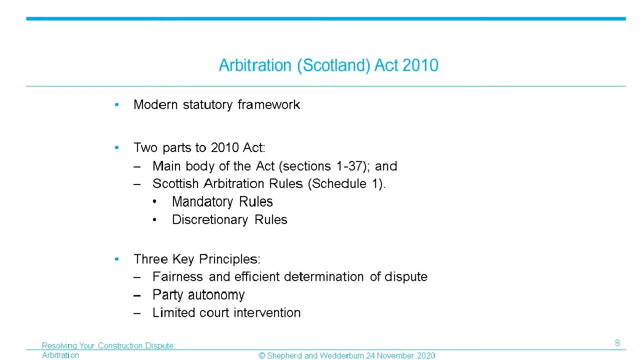 framework for domestic and international arbitration in Scotland. The Act came into force with effect from 7 June 2010,. but it is important to note that the Act applies retrospectively to existing arbitration clauses and contracts concluded prior to the date of commencement. The main body of arbitration is the Act of 2010.. The Act applies retrospectively to existing 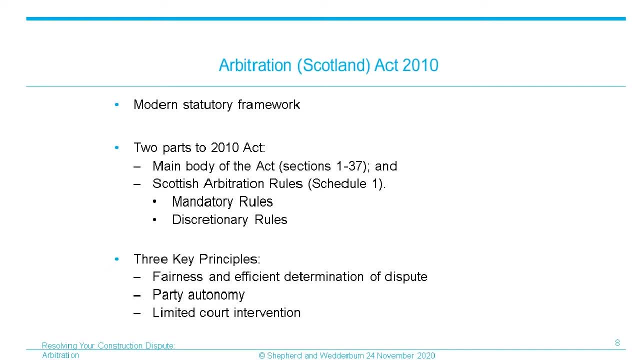 rules and regulations, and the body of the Act runs to 37 sections and regulates the external aspects of arbitration – for example, the enforcement of the arbitral award. Schedule 1 contains the Scottish arbitration rules, which are further subdivided into mandatory rules and discretionary or default rules. The default position is that all of the rules 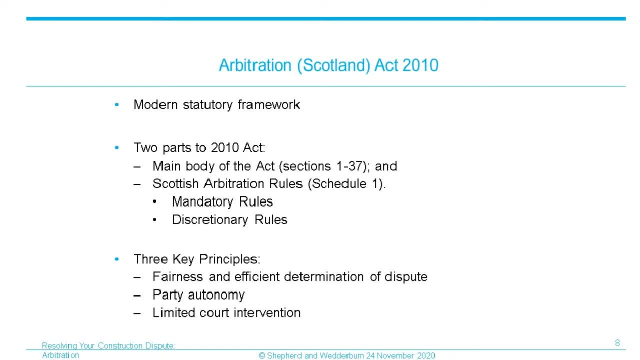 apply. However, before the arbitration commences, parties can agree to opt out of the default rules. This allows parties to shape the procedure to suit their dispute. Section 1 codifies three key principles which have always guided arbitration and which are reflected in the provisions of the Act. 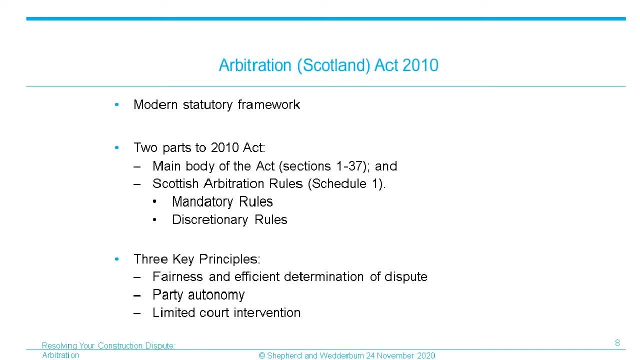 There is a wealth of case law which allows us to predict how these provisions are to be interpreted. The first principle is that the dispute is to be determined fairly and efficiently. The arbitrator is under an express duty to act independently and impartially and to avoid 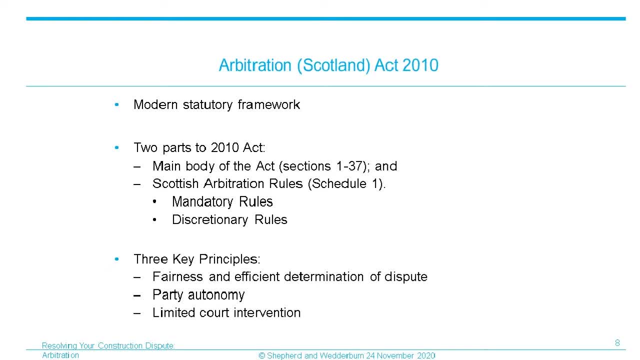 incurring unnecessary delay and expense. The arbitrator is also bound by a duty of competency, and it is a prerequisite to the discharge of their judicial function that they will adequately inform themselves as to the nature and merits of the subject in dispute. The second principle is that the parties have autonomy to influence the 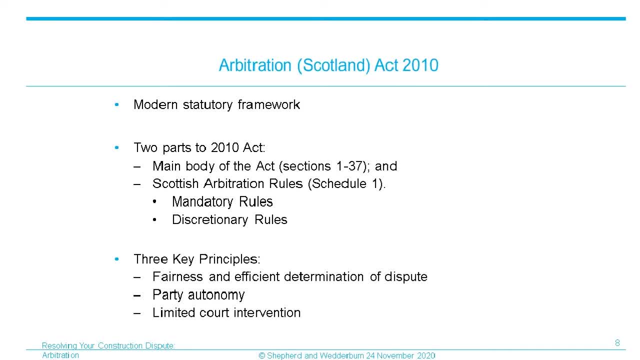 course and procedure of the arbitration. This is reflected in the parties' ability to disapply some of the arbitration rules and thereby influence the way the proceedings are conducted. The third principle follows naturally from the second, and it is a limitation of the court's power to intervene in the arbitration. 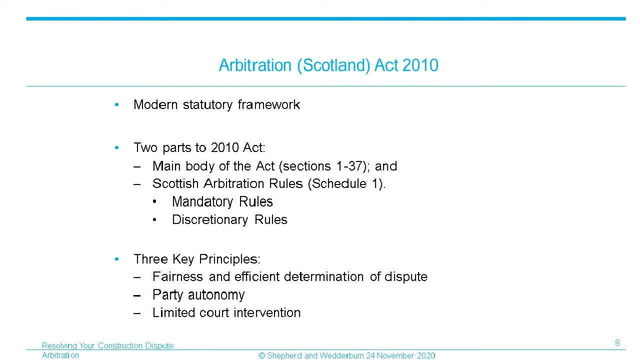 The Act confers on the courts an intentionally limited power of intervention, which therefore empowers arbitration as the parties' chosen process. This is the 3rd principle that follows naturally from the second, and it is a limitation of the courts' power to intervene in the arbitration. 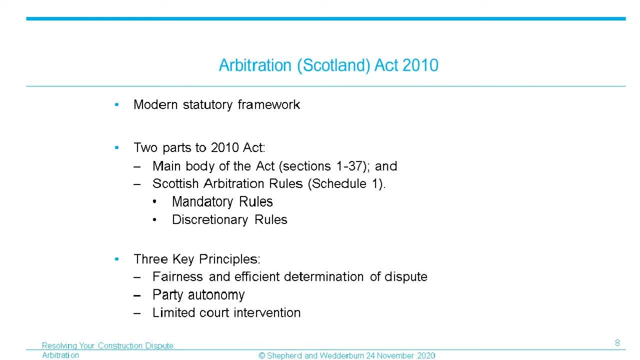 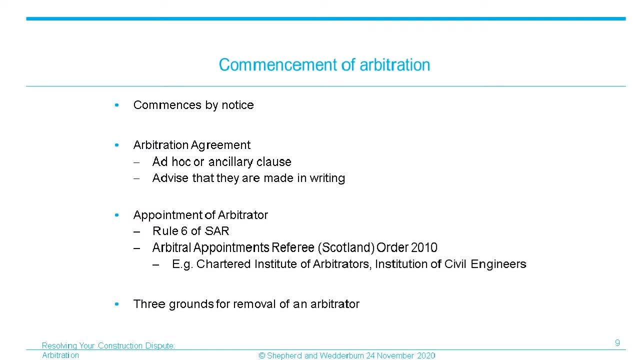 method of dispute resolution. So how does an arbitration begin? Well, a party commences an arbitration by notice to the other party that they intend to submit a dispute to arbitration in accordance with the arbitration agreement between them. This agreement will often set out the procedure by which an arbitrator is to be appointed. This arbitration agreement can be: 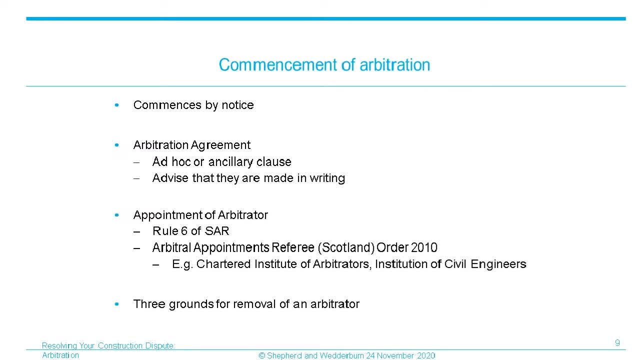 an ad hoc contract of submission. The parties enter into an ad hoc contract of submission where there is an existing dispute between the parties and they agree to submit them to arbitration. However, there is no requirement that the arbitration agreement be a separate, standalone agreement, An ancillary arbitration clause which forms part of another contract. 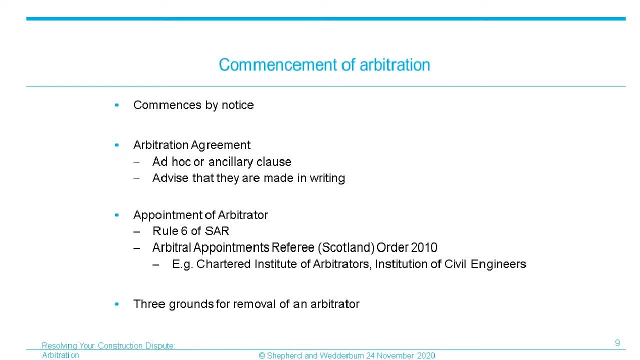 may also be regarded as an arbitration agreement. The Act recognises arbitration agreements which are concluded orally, but this would be invalid where it relates to certain subjects, for example heritable property, and may also lead to problems with enforcement. We would therefore always strongly advise that arbitration agreements are made in writing. 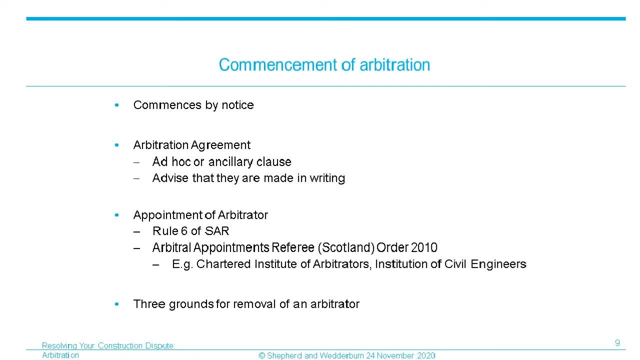 The default rule under the Scottish arbitration rules is that the parties must jointly appoint an arbitrator within 28 days of either party requesting an arbitration agreement. If not, either party may seek the appointment of an arbitrator by an arbitral appointments referee. There are a number of bodies that may act in this capacity. 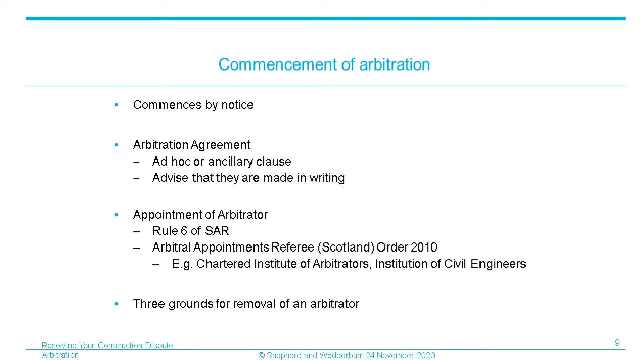 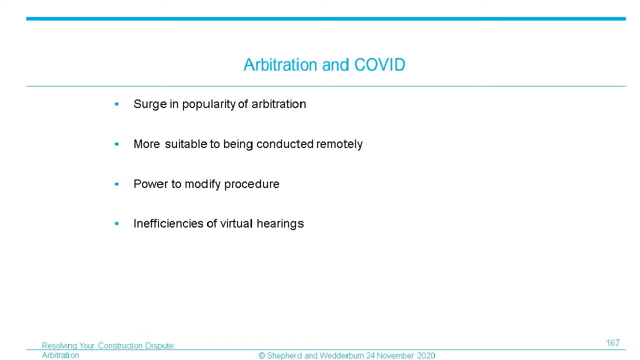 Finally, acting under this rule, the tribunal may order the rectification of a deed or a document exist in in-person hearings. These should be borne in mind, and borne in mind that it will take time to prepare, over and above all the other preparations that are required. 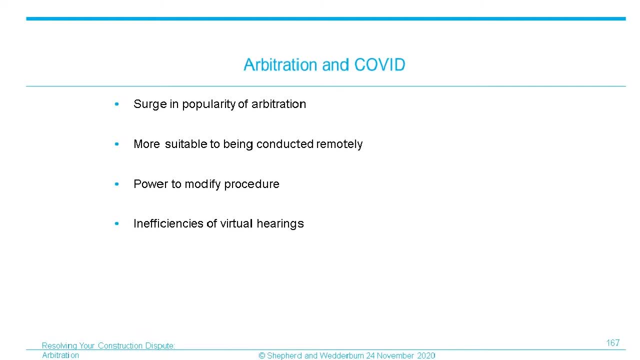 should the tribunal decide that there should be a hearing and that it is to be a virtual one? We have now come to the end of this webinar, which we hope has been useful to you, and we still have a few minutes to answer any questions. If you haven't already done so, please type your questions. 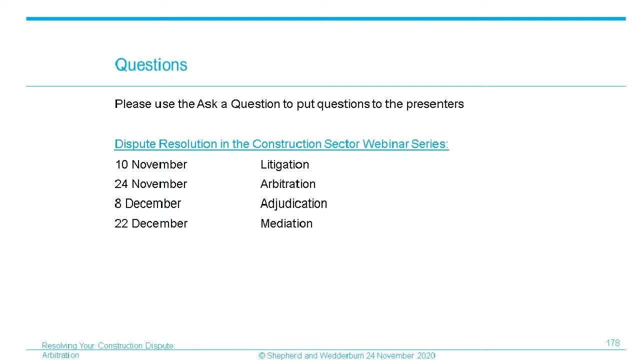 into the chat box now. While you're doing that, I would just like to remind you that the next webinar in this series will be available on Tuesday, the 8th of December 2020, and will cover adjudication in the construction sector. If you would like to sign up for this webinar, please. 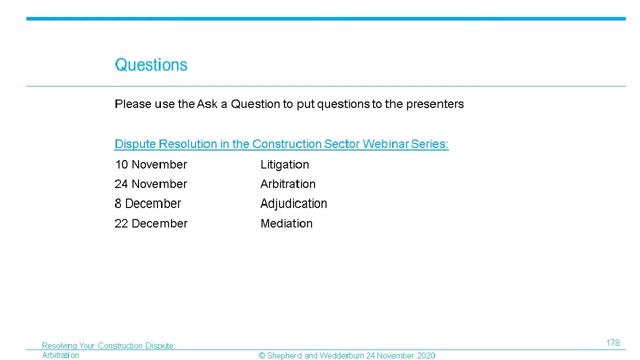 visit the events section of our website. You can listen live or can register to the website. Thank you, Be sent a recording of the webinar and to listen to that at your leisure. Thanks, Lisa, Let's have a look at the questions. Okay, so there's a question about the uptake of 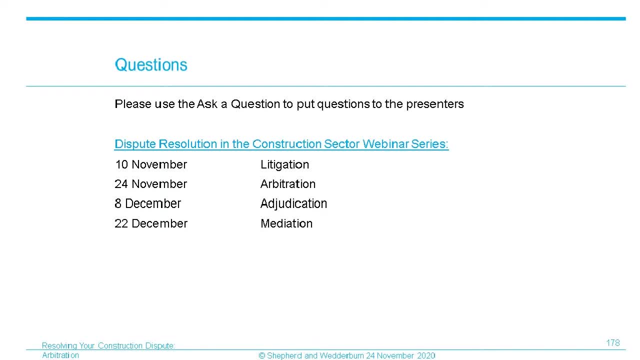 Scottish arbitrations since the 2010 rules. That's a very good question. So it's been about a decade since the Scottish arbitration rules came into force and the question is whether there's been an increase in the uptake, and I think our answer to that would be yes, Yes, 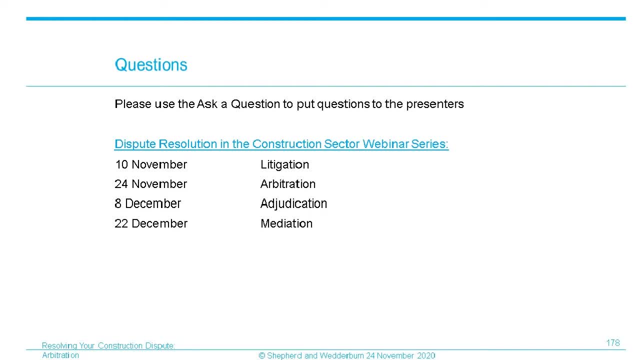 there has been an increase in arbitration and there has been an increase in the uptake been it's increasing. As we described at the beginning of the webinar, there were historical problems with arbitrations that put a lot of people off of them, But I think since the 2010. 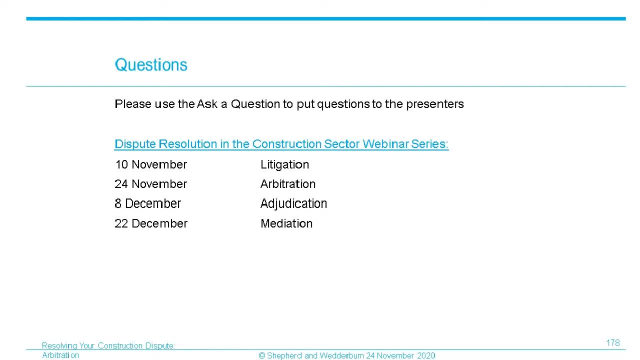 rules have come into effect, people have become gradually much more comfortable with Scottish arbitration, So we're not starting from a particularly high base. There's not many arbitrations before 2010.. And obviously at that time the Court of Session was pretty well known. 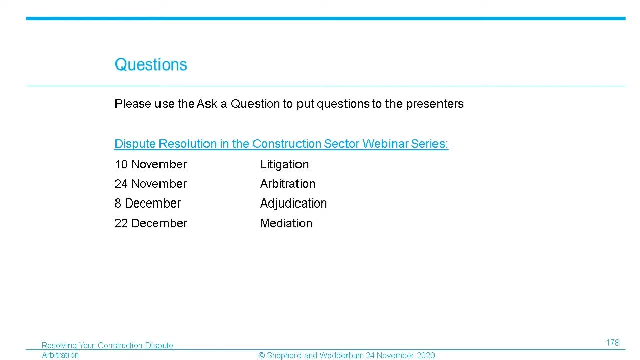 and trusted. But I think there has been an increase as the comfort of the rules and arbitration process in Scotland has increased And, as we mentioned, certainly in the last year with the coronavirus circumstances that really has made people think about how they tackle their disputes. 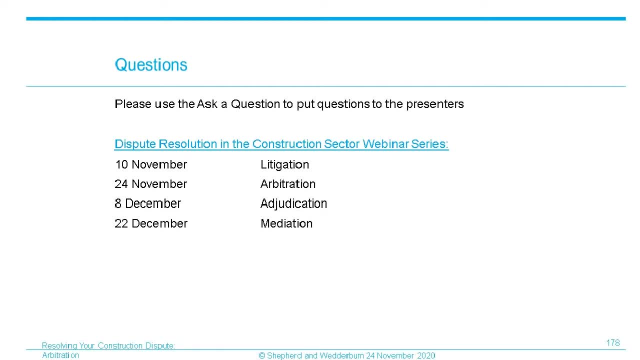 and whether the public courts are the best place or whether really, I suppose, making their own arrangements through a private arbitration can be better. So I think they've probably increased even more over the last nine months than before. So, yes, certainly the uptake is. 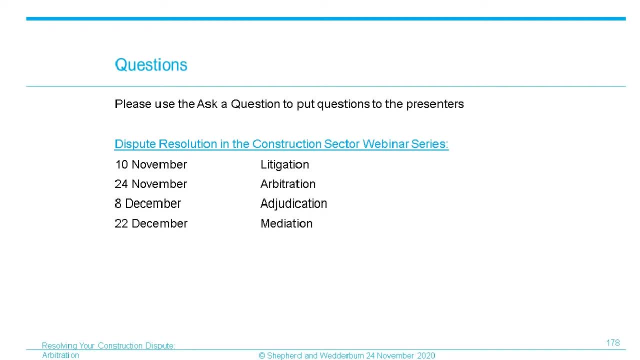 increasing. Now let's have a look. I think we've got time for one more question, So this is a good one, actually a fairly classic question, which is: how would you decide between, for example, the Court of Session or litigation versus arbitration? There's obviously pros and cons. 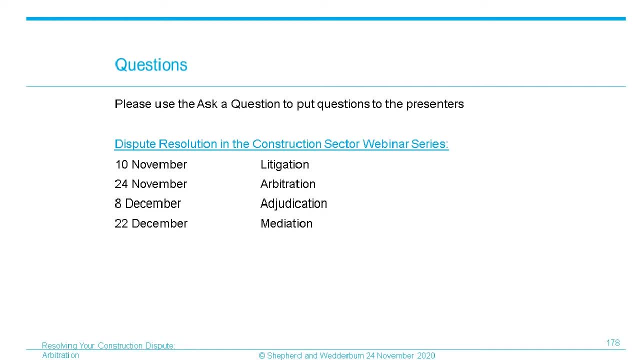 to both. I think the first part of that answer is obviously: first of all, we're going to look at your contract, because it's It's very usual that your contract will tell you- or it will have already been decided- what your 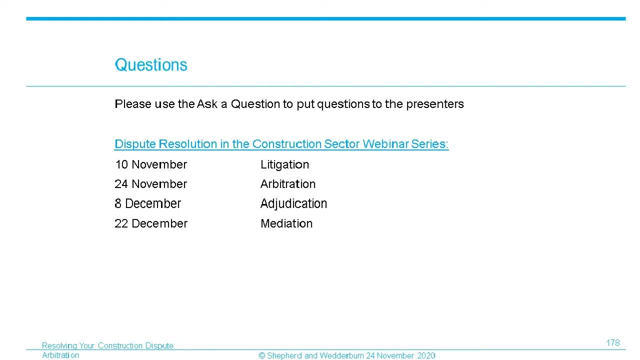 dispute resolution route is So you might have no choice: whether to go to court or whether to arbitrate. In terms of if you either do have a choice or if you're at the stage of, I suppose, agreeing your dispute resolution process in a contract, there's certainly pros and cons to both. 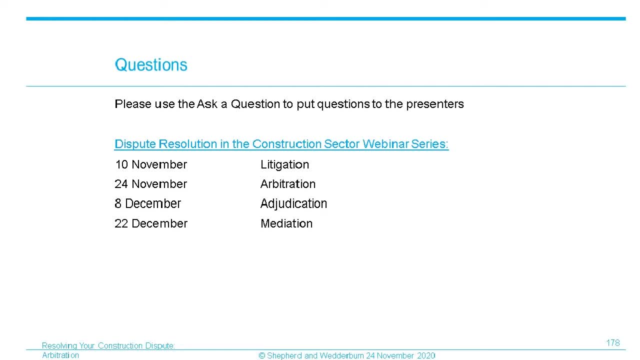 And we do find that it depends on the parties and people can have particular preferences, but certainly the main pros for arbitration that comes out in our discussions with clients is the privacy and confidentiality aspects. Having a dispute resolved out of the public gaze has a 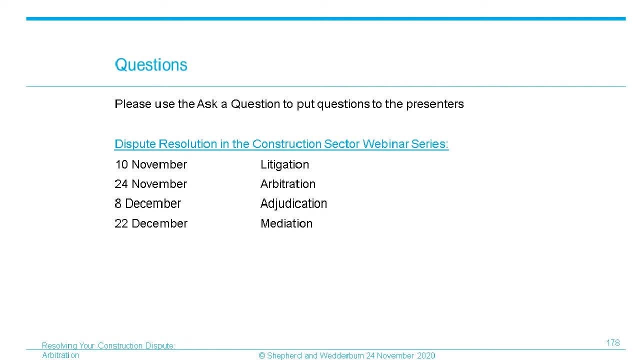 lot of attraction for commercial clients And I suppose also sometimes speed, particularly if it's under quite good rules, then arbitrations can be quicker and there's certainly more control over the speed than the And perhaps a slight vagueness of timescales in the court of session where, for example, the timescales 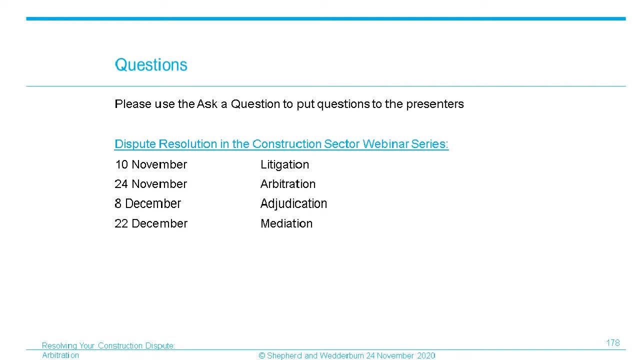 might really depend on how busy the court is at any particular point. However, some people do prefer the courts. Even commercial clients, you know, and certainly others can just look to have their day in court. They may actually appreciate the public side of court and perhaps might have more trust in. 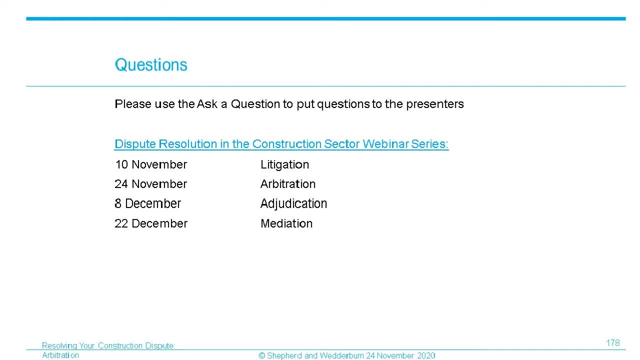 I suppose public opinion, And so I think it's really important that you have that kind of public justices and more confidence in that process than a private arbitration practice. So certainly those people who have less experience of arbitration might be a little bit more. 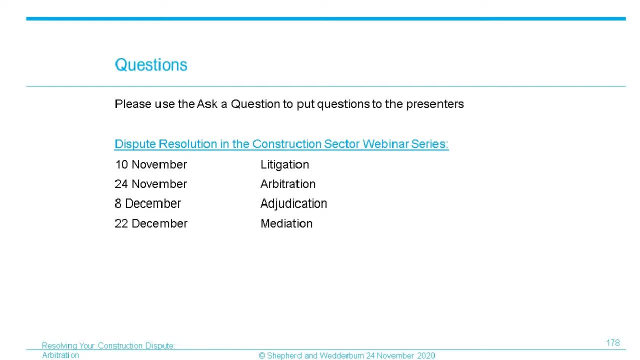 sceptical about it. Both work fine, though in the end really, and our experience is that both tend to- in the round, I suppose, tend to deliver justice. So it probably will depend on clients or your particular circumstances and preferences. I think that's all I would say on. 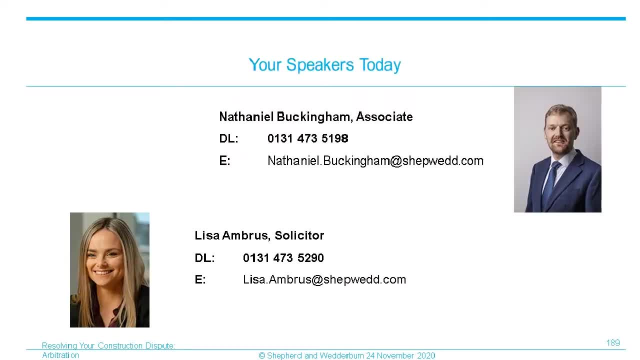 that. So I think that's probably all the time we have. If there's any other just looking at the questions, if there are any others that we've not answered, we'll come back after the webinar and answer them. We do hope that you've enjoyed this webinar, which has been recorded and will be